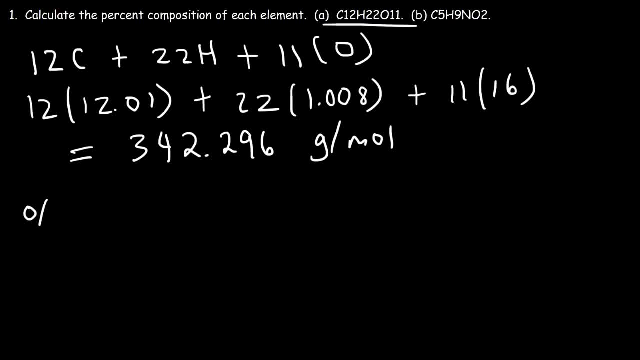 So that's the molar mass of the entire thing. Now, if you want to find the percent by carbon, you need to take the molar mass of all 12 carbon atoms and divide it by the total and then multiply it by 100%. 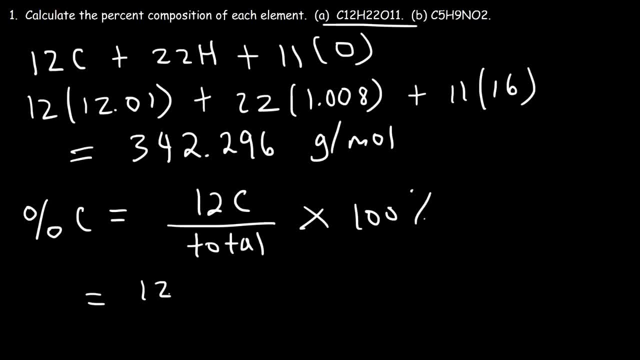 So each carbon is 12.01.. That's the atomic mass. The total molar mass is this number that we have, 342.296.. And then we're going to multiply it by 100%. So that's the total molar mass. 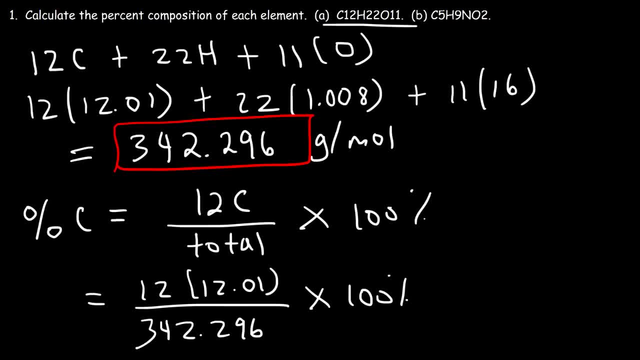 And then we're going to multiply it by 100%. So 12 times 12.01, that's 144.12.. Divide that by 342.296, and then take that result and multiply it by 100% And you should get 42.1%. 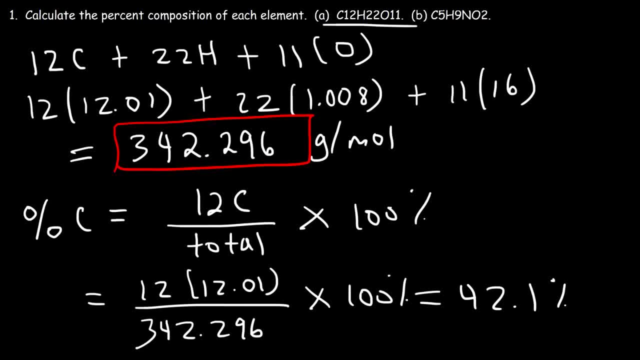 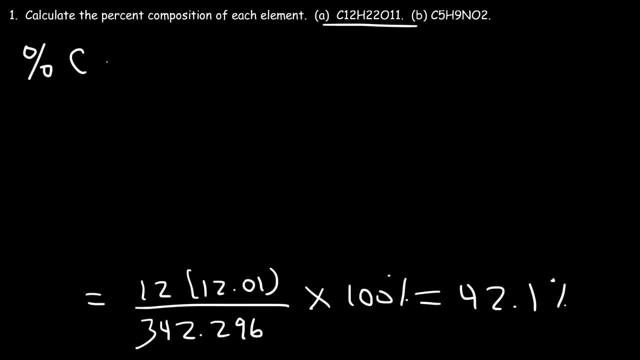 So that's the percentage by mass of the carbon atoms in sucrose. Now I'm just going to rewrite the answer on the top so we can reference it later. So it's 42.1%. Now let's do the same thing with hydrogen. 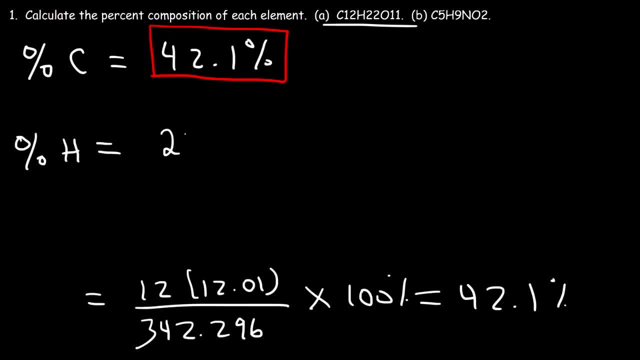 So we need to take the mass of all the hydrogen atoms- There's 22 of them. Each has an atomic mass of 1.008.. And divide it by the same total mass for the entire compound, which is 342.296.. 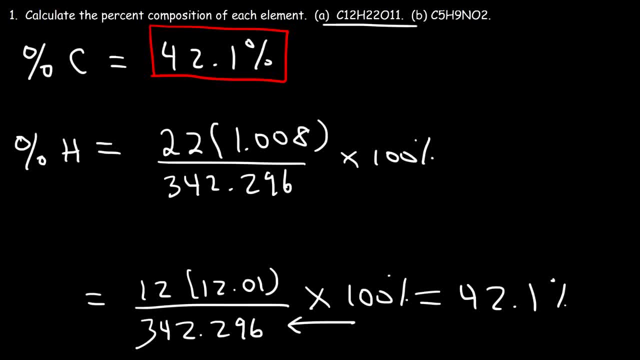 And then multiply everything by 100%. So 22 times 1.008, that's 22.176.. And then divide that by 342.296.. And then multiply by 100. This will give you about 6.5% if you round it. 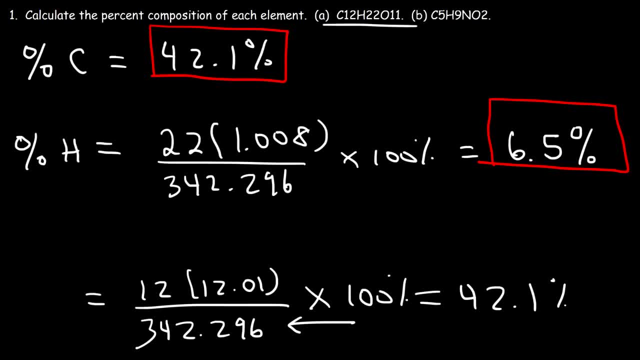 Now let's do the same thing with oxygen. So in sucrose there are 11 oxygen atoms, each with an atomic mass of 16. Then divide it by the total molar mass, 11 times 16, that's 176.. 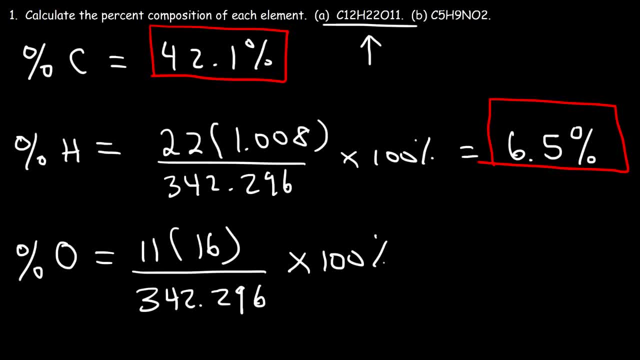 And then divide it by the molar mass and multiply it by 100. You should get 51.4.. 51.4.. So that's the percent by oxygen, or the percent by mass of oxygen. Now, if you add up 51.4,, 42.1, and 6.5, this will give you 100%. 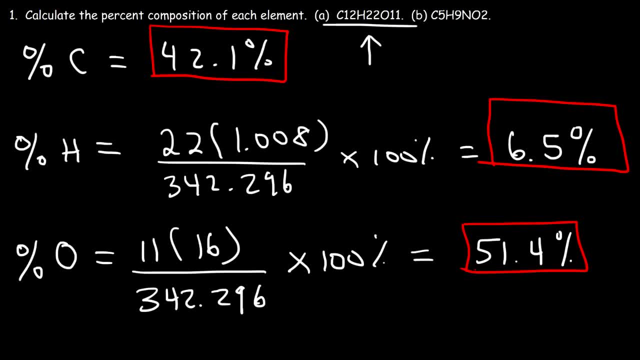 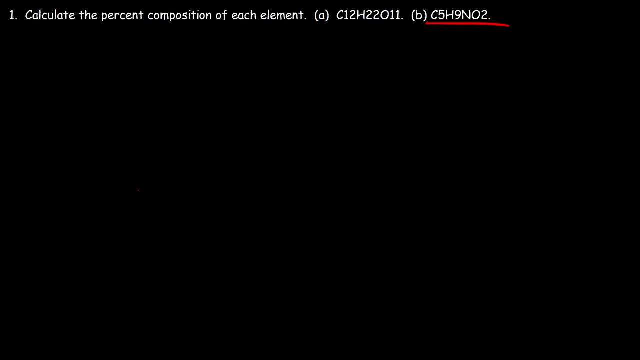 That's how you can tell if you did everything correctly. So now let's move on to our next example. Let's calculate the percent composition of every element in C5H9NO2.. So first let's find the molar mass of the entire compound. 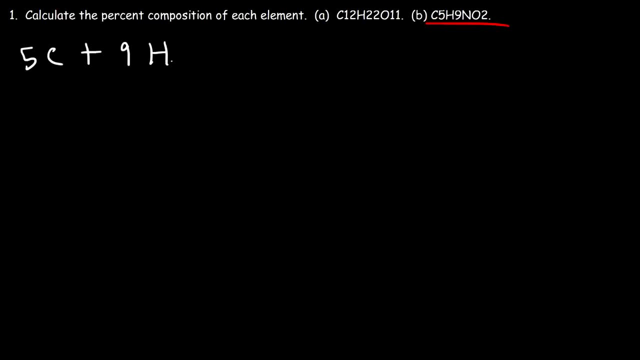 So we have 5 carbon atoms, 9 hydrogen atoms, 1 nitrogen atom and 2 oxygen atoms. Now let's replace carbon with its atomic mass of 12.01.. H is 1.008.. Nitrogen: 14.01.. 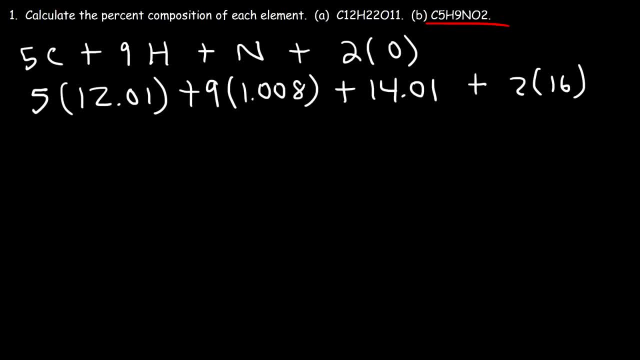 And oxygen, it's 16.. Now, 5 times 12.01 is 60.05.. 9 times 1.008, that's this number, And then 2 times 16 is 32.. So let's add everything. 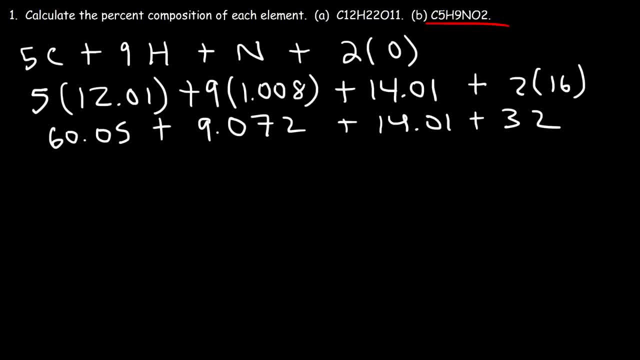 So the total molar mass is 115.132 grams per mole. So now that we have that, we can calculate the mass percent of every element. So let's start with the percent of carbon. So it's going to be the 5 carbon atoms which we can see that it has a mass of 60.05.. 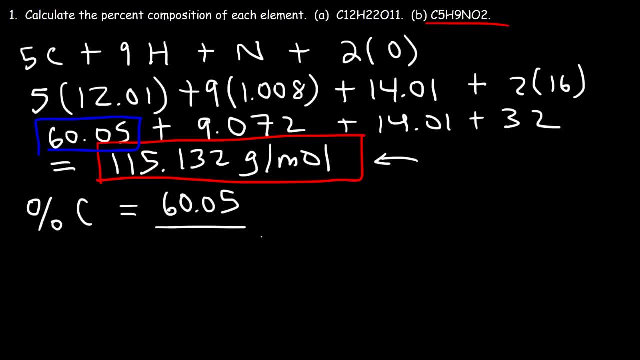 Divided by the total molar mass of 115.132 times 100%, So it's 52.16% bicarbon. Now let's move on to the percent by hydrogen, or the percent of hydrogen, rather. so it's going to be. 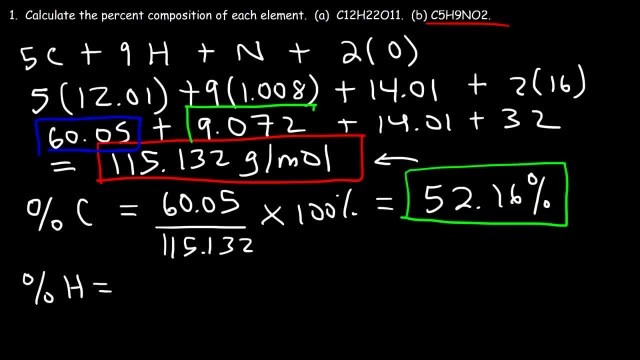 the nine hydrogen atoms, which has a mass of nine point zero, seven, two, divided by the same total molar mass of 115 point one, three, two times 100%, and so that's going to be about seven point eighty eight percent. now let's do the same for 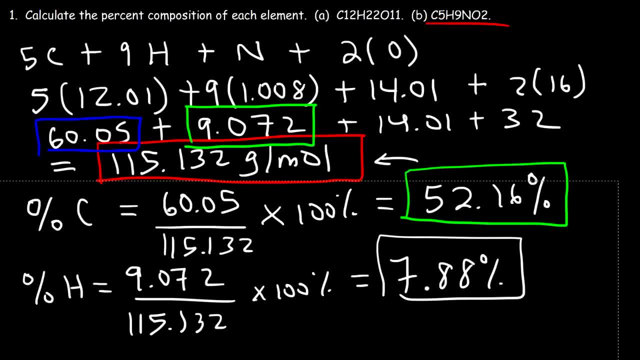 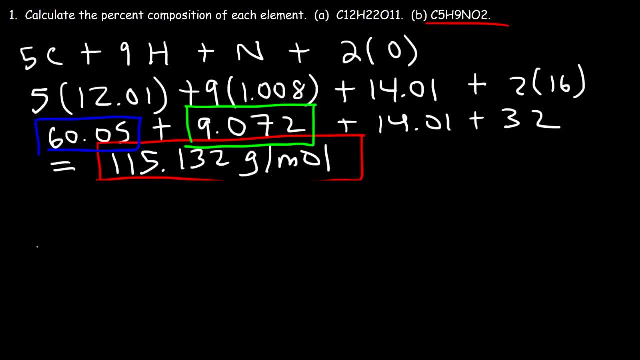 the remaining two elements. so let's move on to nitrogen. so we have the mass of nitrogen, which is a 14.0 one divided by the total times 100. so once you do this a few times, it becomes second nature. your automatically get the hang of it. 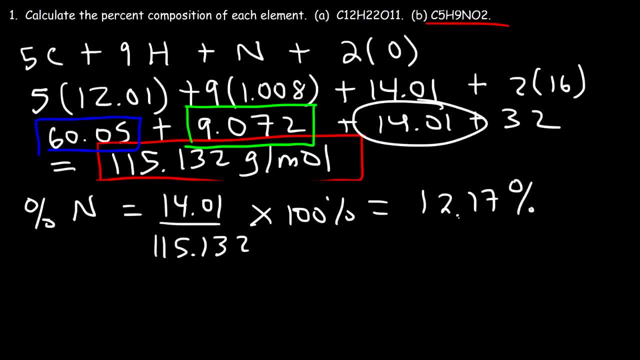 so it's 12.1 percent for nitrogen. now let's move on to oxygen, the last one. there are two oxygen atoms, and so the molar mass of those two oxygen atoms is 32, and, just as we've been doing before, we're going to divide it by the total, so nothing has changed except the top. 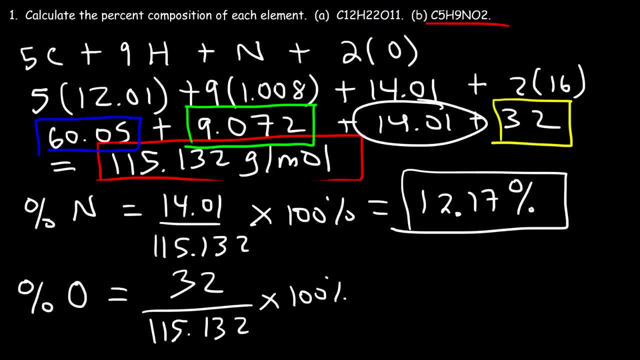 number and I got twenty seven point seven, nine percent for the value of oxygen. so that's the mass percent of oxygen in that compound. so now you know how to find the percent composition of every element within a molecular compound. and that's it for this problem. number two: which of the following compounds contain the greatest? 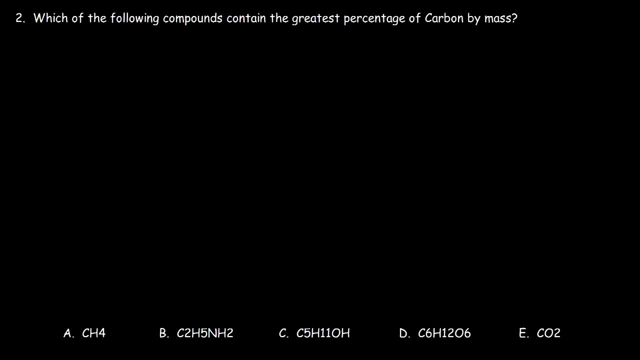 percentage of carbon by mass. is it going to be a, b, c, d or e? well, the most simplest way to find the answer is to determine the percentage of carbon for each compound. let's start with ch4. so the percent of carbon is going to be. the mass of carbon is only one carbon atom and we know the atomic. 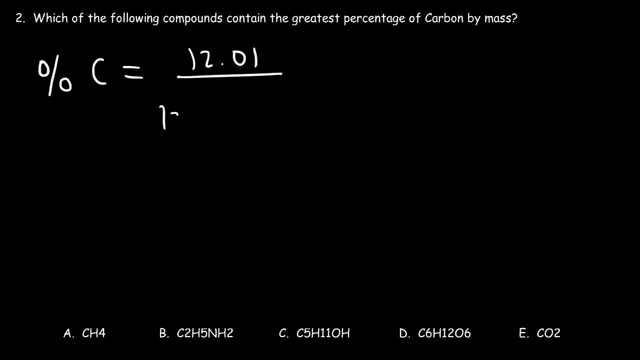 mass is 12.01 divided by the total, which is the mass of carbon plus the four hydrogen atoms, and then we're going to multiply by a hundred percent. now let's find the molar mass of ch4. let's start with that first, so 12.01. 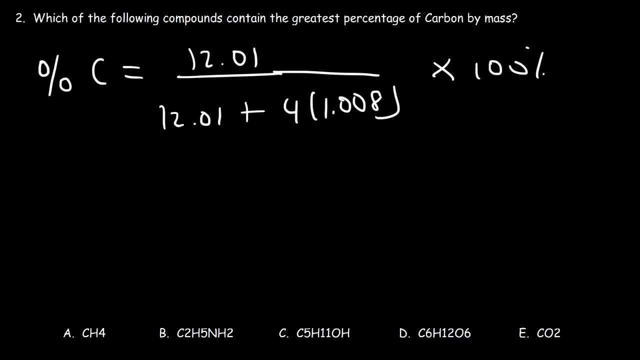 plus four times 1.008, that's 16.042. let's multiply everything by a hundred percent, so this is 74 point eight, seven percent mass by carbon. so let's look at the second example. let's see if there's anything that can top that. so for B there are two. 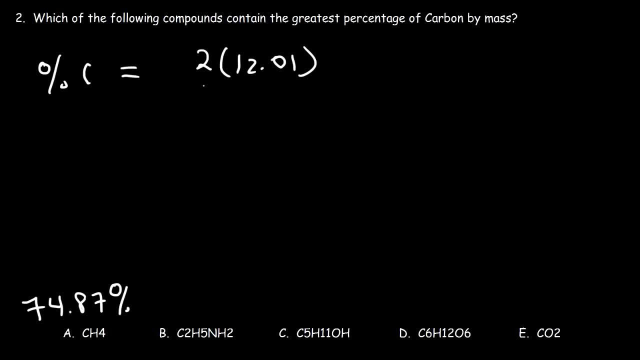 carbon atoms. so it's two times 12.01 divided by the total, which will be the two carbon atoms, and there's a total of seven hydrogen atoms. five plus two is seven, and we have a nitrogen atom as well. so let's calculate the molar. 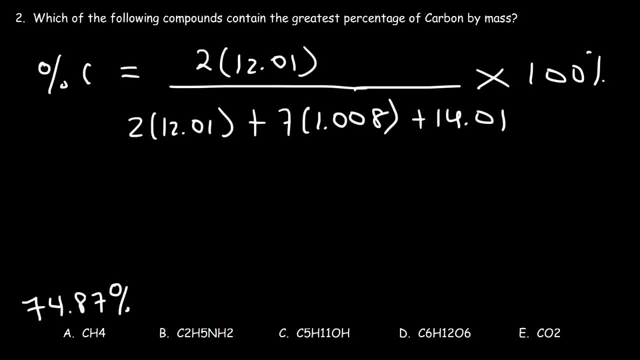 mass first. so for the molar mass I got 45.086. two times 12 that's going to be 24. So the percentage is 53.3%. So we can eliminate answer choice B. So far A is the highest. Now let's move on to part C. 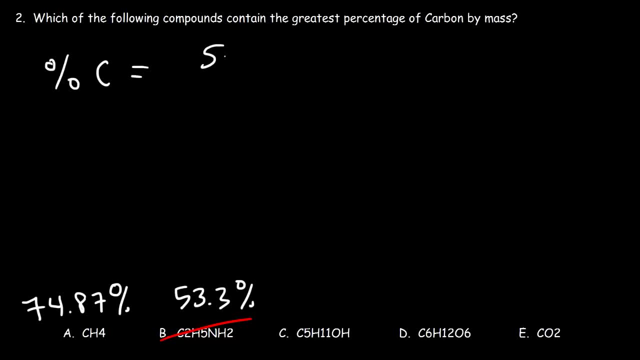 So this time we have 5 carbon atoms, so it's going to be 5 times 12.01.. Divided by those 5 carbon atoms and there's 12 hydrogen atoms, not 11, and we have an oxygen atom. 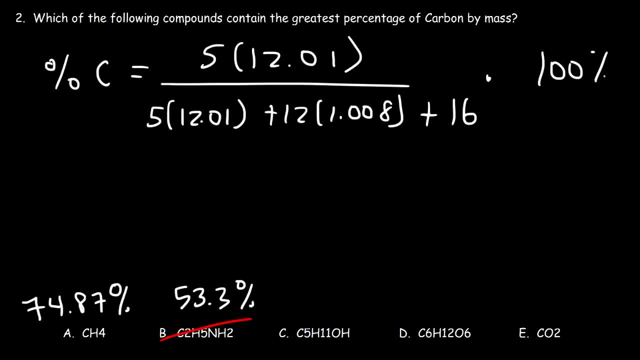 So let's multiply that by 100%, So 5 times 12.01.. That's going to be 60.05.. And the total molar mass of C5H11OH is 88.146, if I did that correctly. 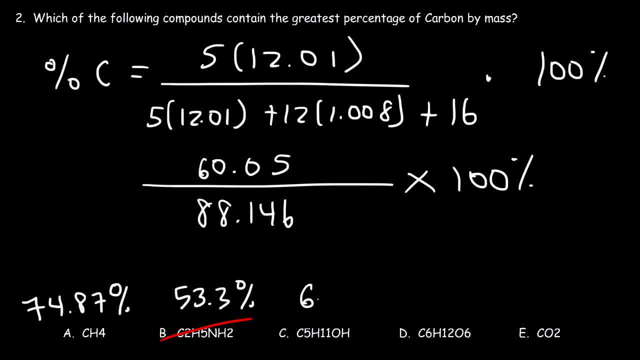 Okay, of carbon in this sample is 68.1%, which is still less than 74,, so we can get rid of that. Now let's move on to Part D. So we have six carbon atoms, this time divided by everything else. 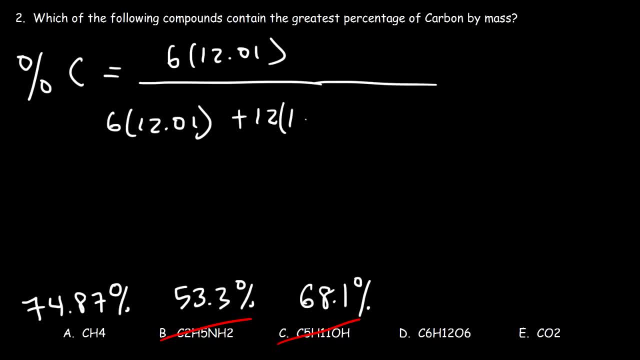 There's 12 hydrogen atoms and 6 oxygen atoms. 6 times 12.01, that's going to be 72.06.. And the molar mass of C6H12O6, that's 1.6.. 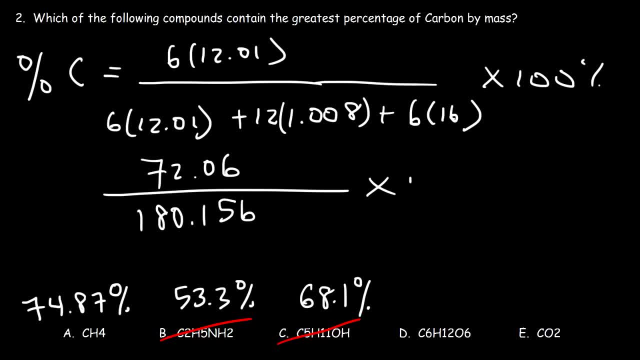 So that's 180.156.. So the percentage is about 40% carbon. Now the last thing we need to check is carbon dioxide, which is probably not going to be more than 50%, probably a lot less. So we have one carbon which is 12.16.. 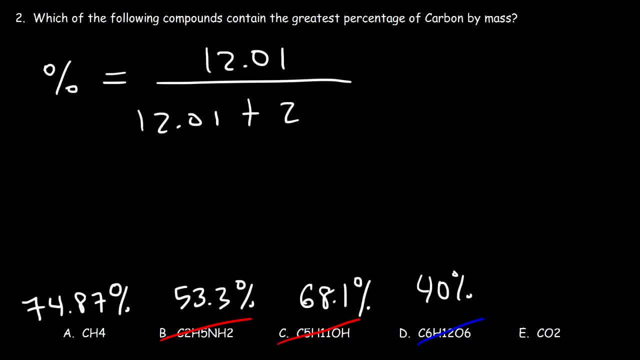 So that's going to be about 40.01,. divided by the total, The molar mass of CO2 is 44.01.. So you should get 27.3%, which is the lowest. So therefore the answer is A. 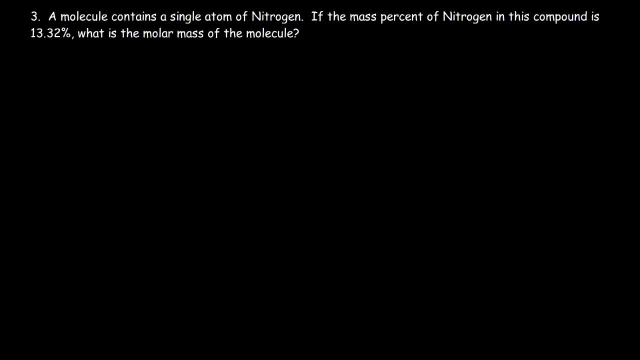 Number three: a molecule contains a single atom of nitrogen. If the mass percent of nitrogen in this compound is 13.32%, what is the molar mass of that molecule? So how can we figure this out? Well, let's start with a formula. 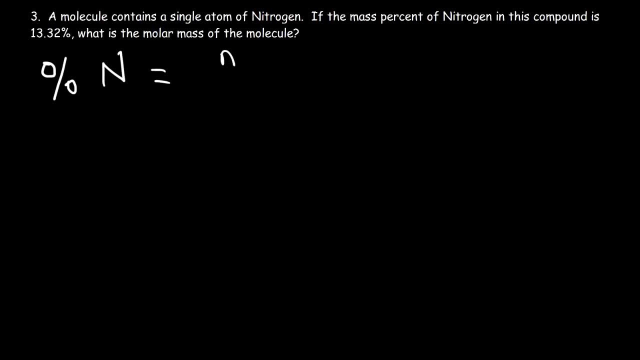 The percent of nitrogen is going to equal the mass of nitrogen divided by the total molar mass, multiplied by 100%. So we have the percentage of nitrogen in this compound. It's given to us as 13.32%. Now we know that there's a single nitrogen atom.